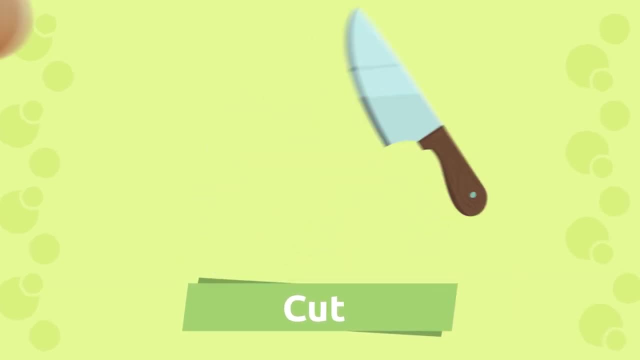 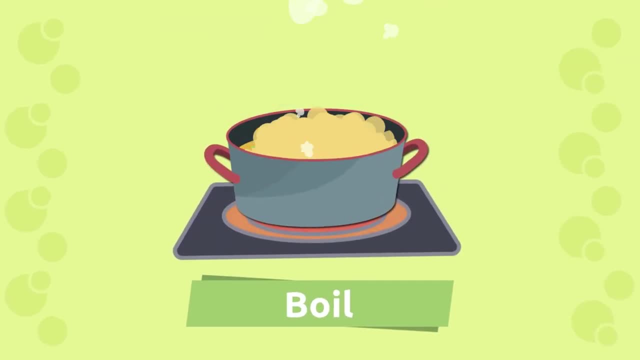 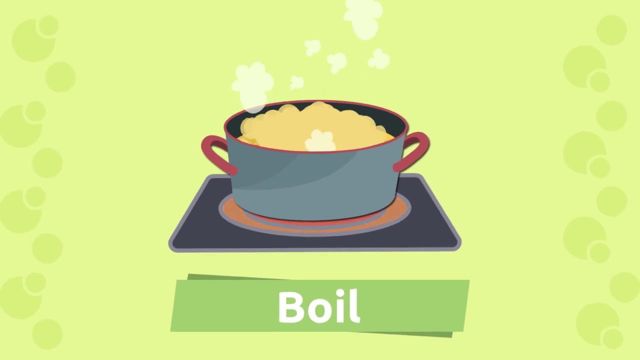 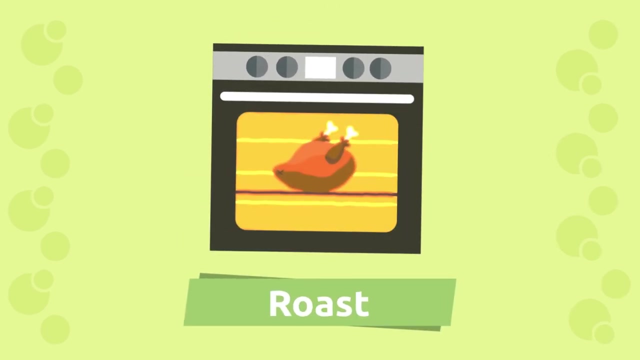 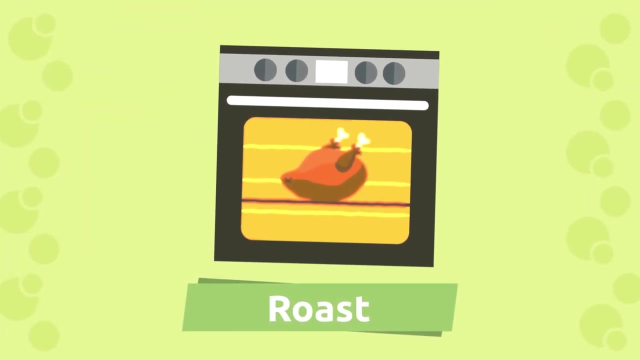 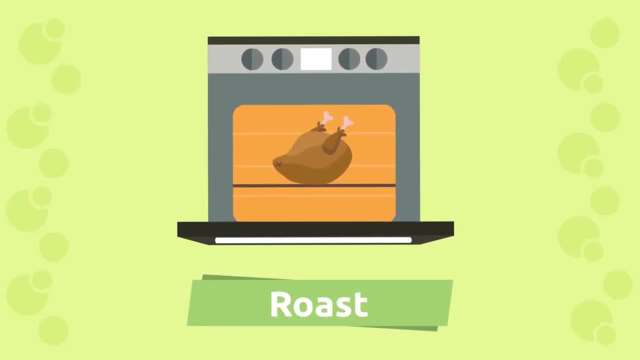 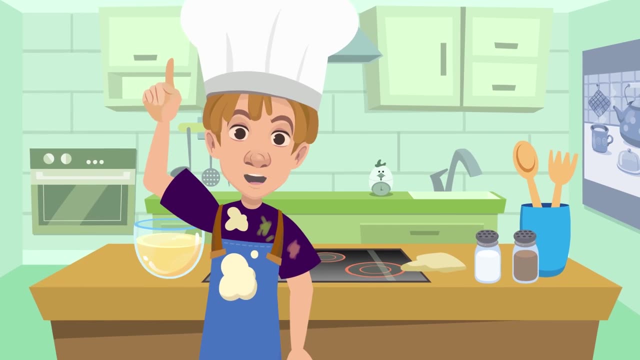 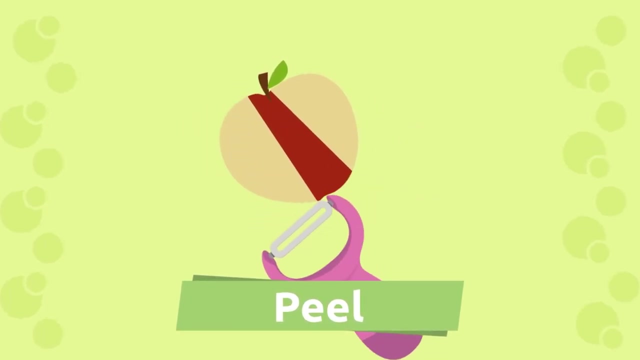 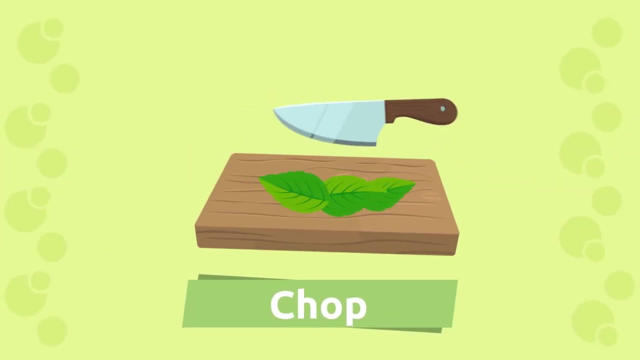 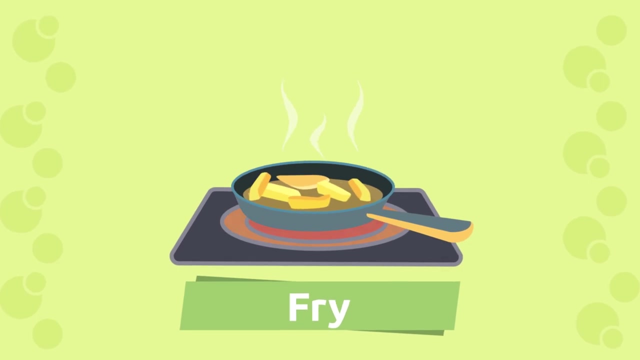 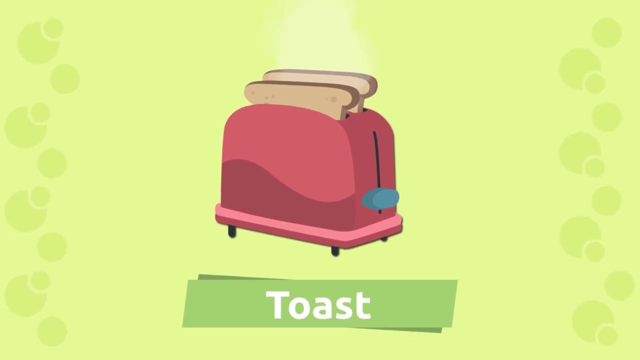 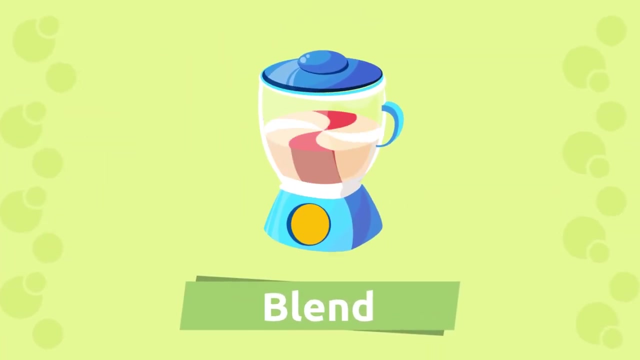 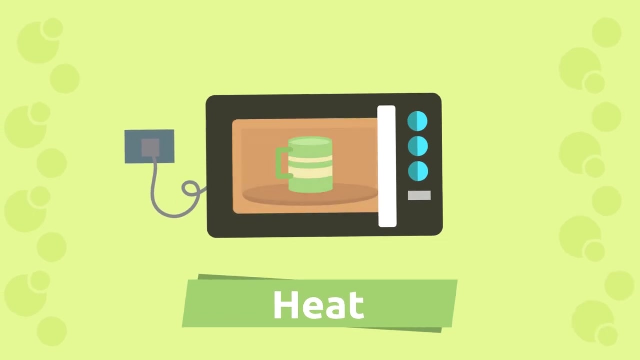 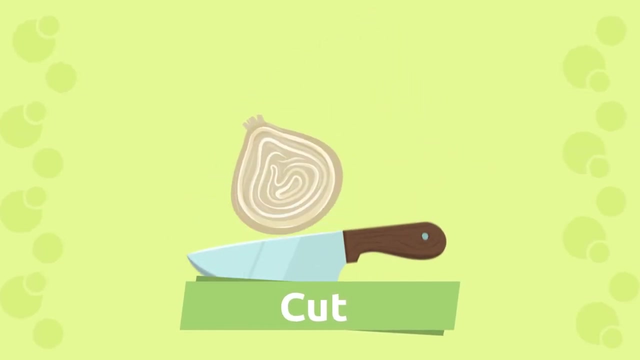 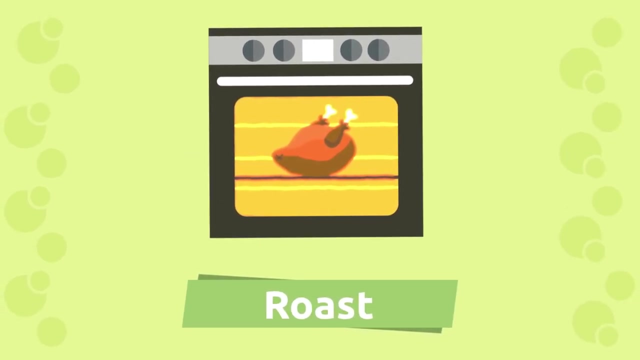 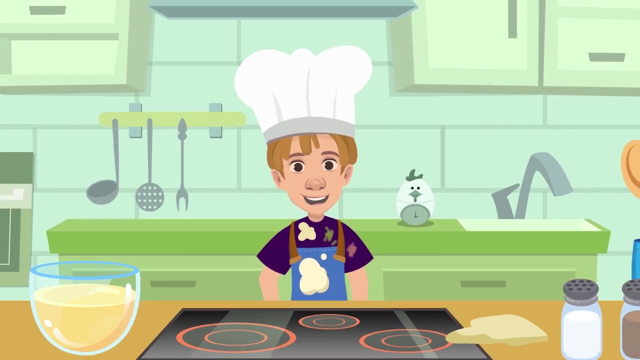 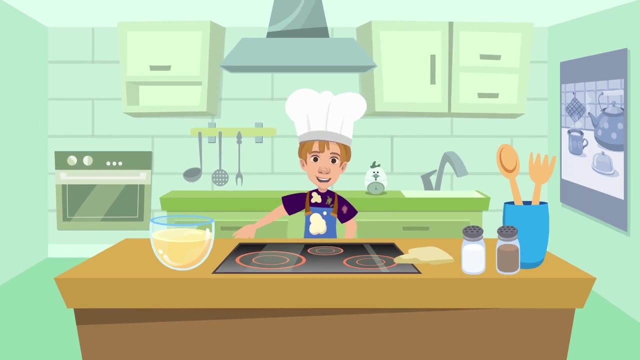 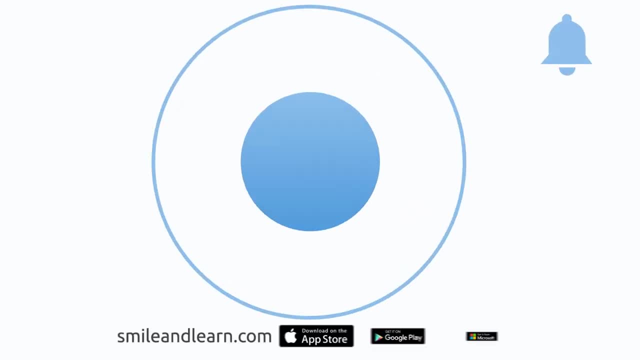 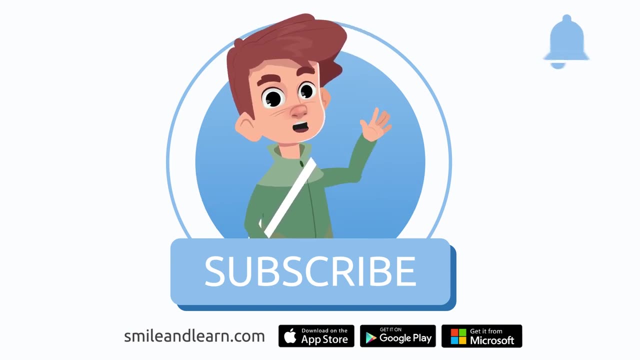 We've learned so much in just one video. Did you know there are many more videos? Imagine how much you could learn. Subscribe to the Smile and Learn educational channel to learn and have fun at the same time.